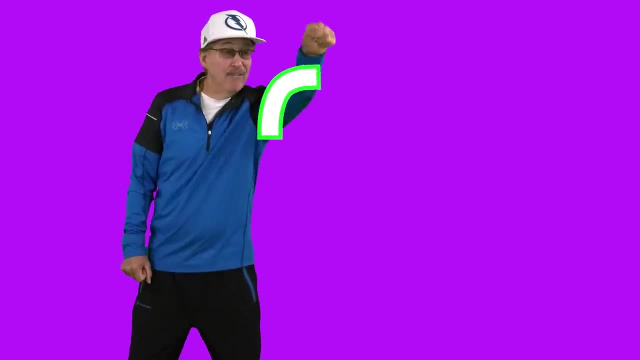 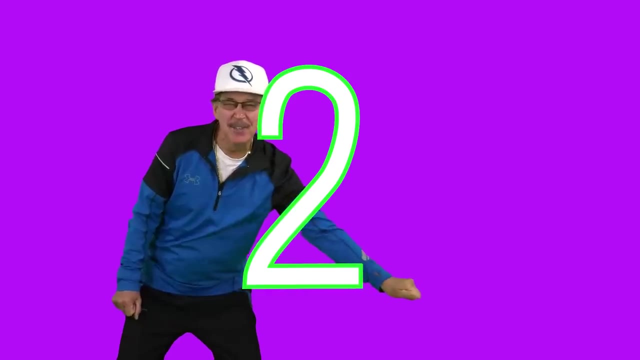 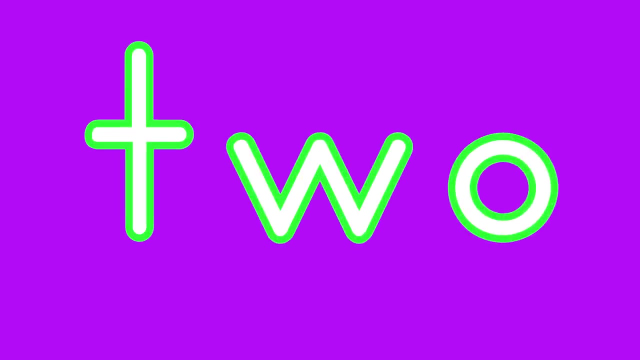 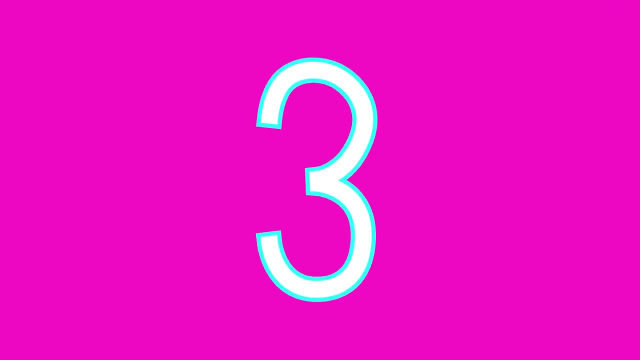 It's number two. Make half a heart, Give it a shoe. Top to bottom. It's number two. T w o Number two. T w o, Number two. This is number three. This is number three. This is number three, And you write it like this: Half round a tree. 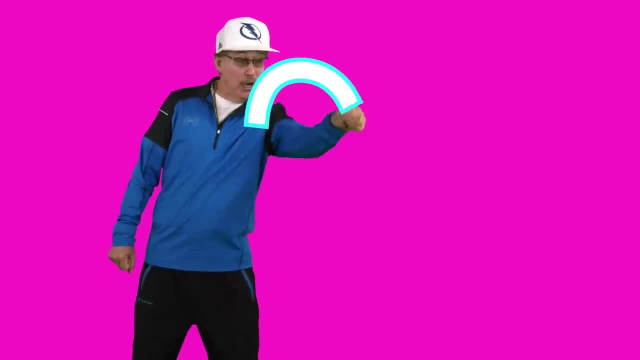 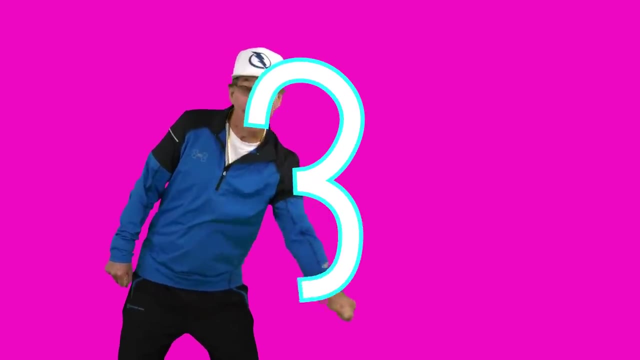 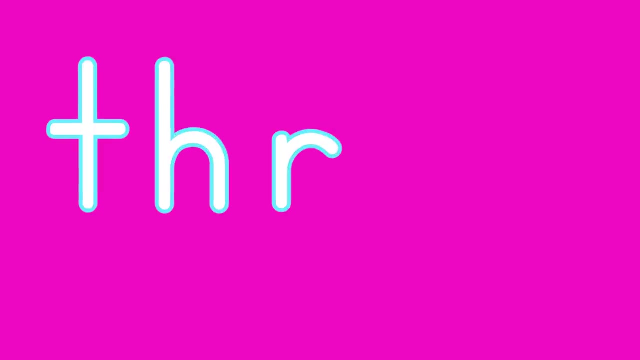 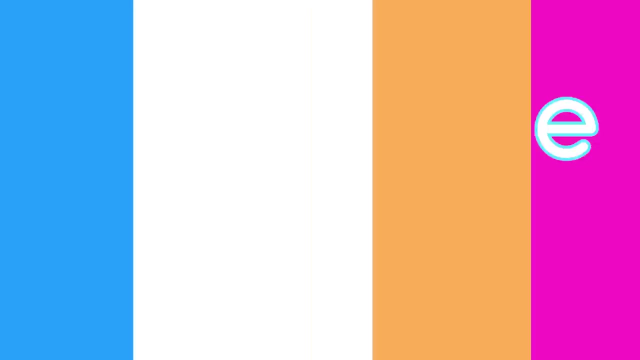 Half round a tree. Curve it, curve it. It's number three. Half round a tree. Half round a tree. Curve it, curve it. It's number three. T h r e e, Number three. T h r e e, Number three. This is number four. This is number four. 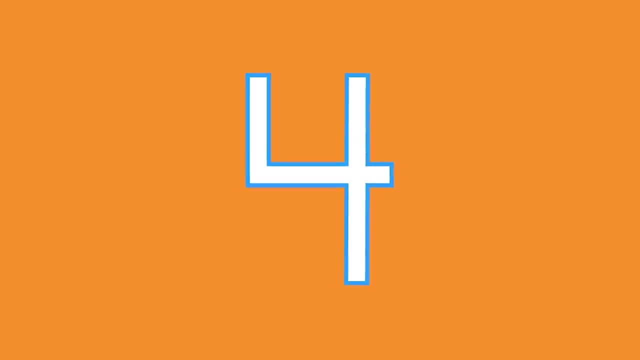 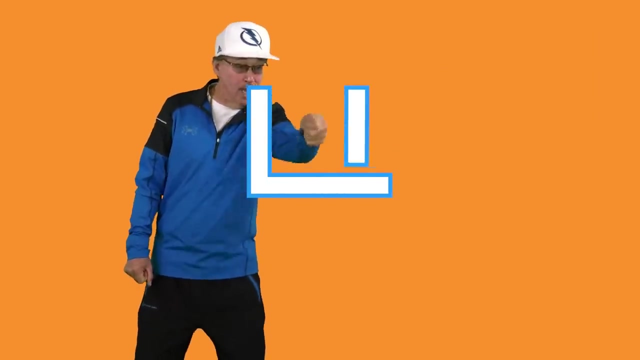 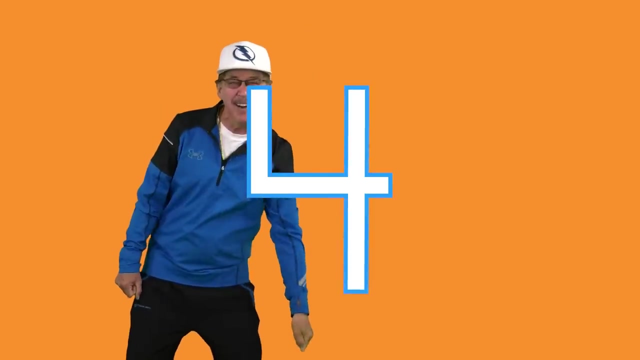 This is number four, And you write it like this: This is number four, And you write it like this: Down and over and down, some more, All straight lines. It's number four. Down and over and down, some more, All straight lines. It's number four. F o u r. 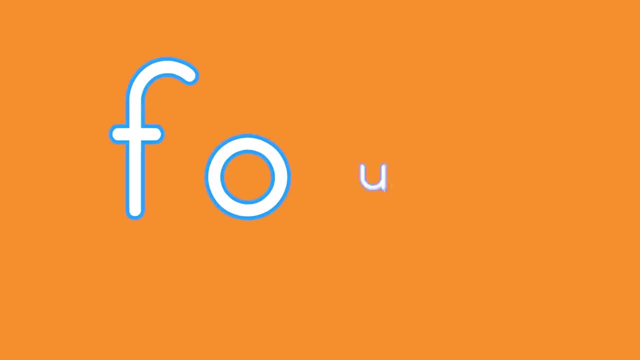 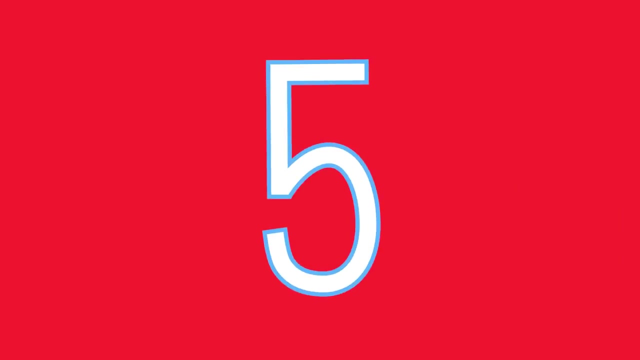 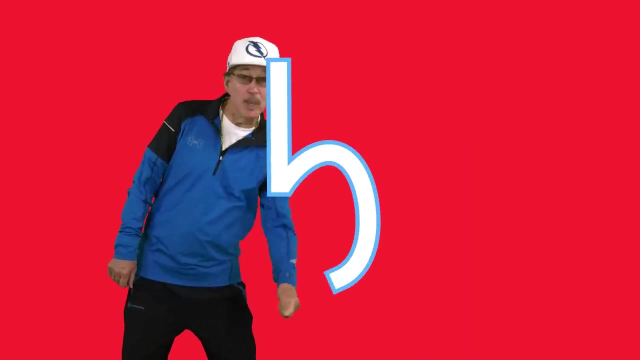 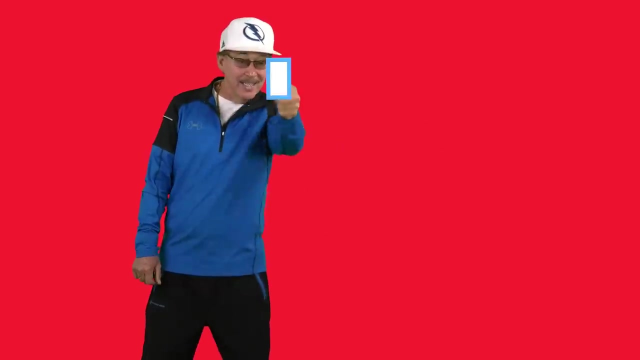 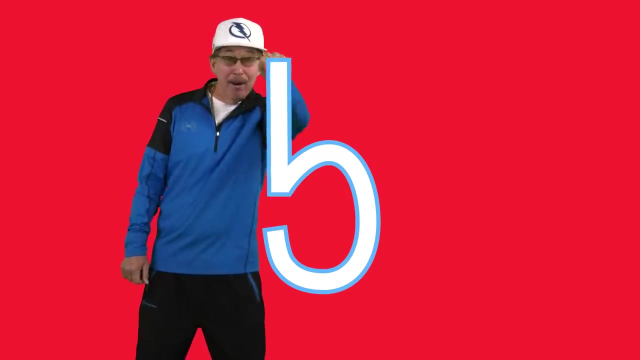 Number four: F o u r Number four. This is number five. this is number five. this is number five. And you write it like this: Down and around with a flag on high, Every time it's number five. Down and around with a flag on high, Every time it's number five. 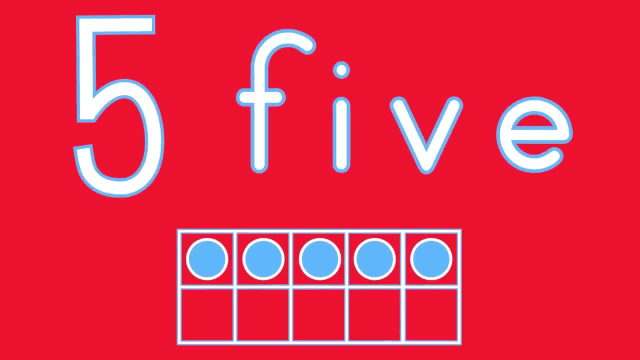 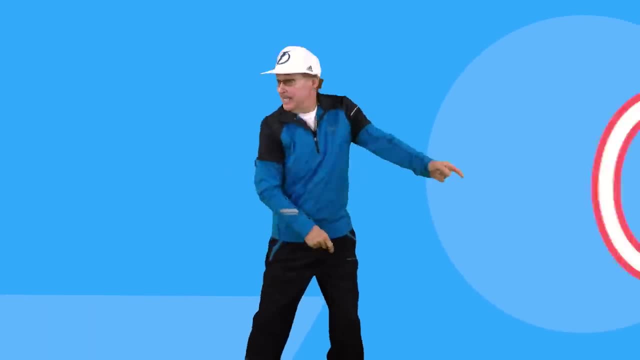 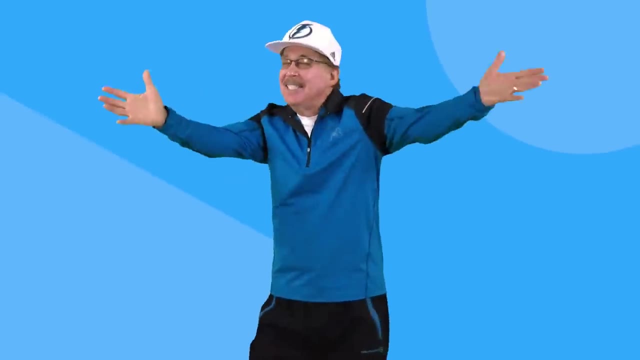 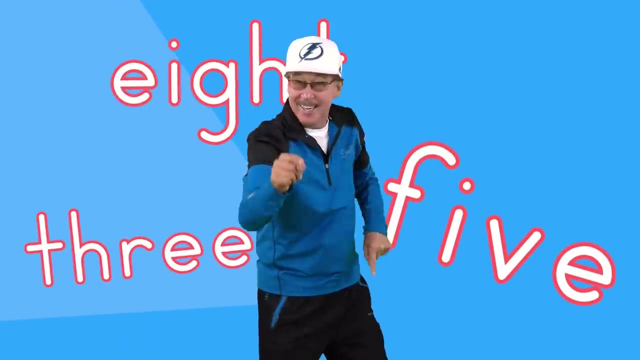 F-I-V-E- number five. F-I-V-E- number five. Let's learn our numbers zero to ten, Learn how they look and how to write them. my friends, Let's learn our numbers zero to ten. Even learn how to spell them again and again. This is number six. this is number six. 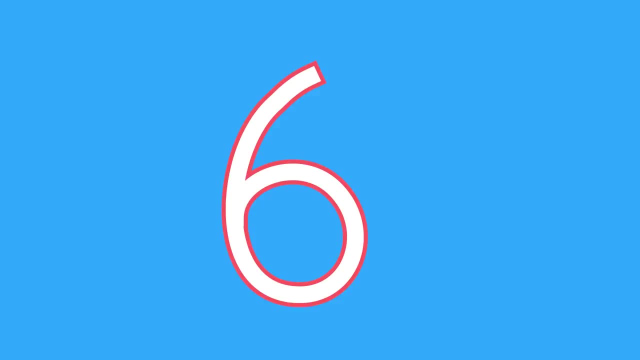 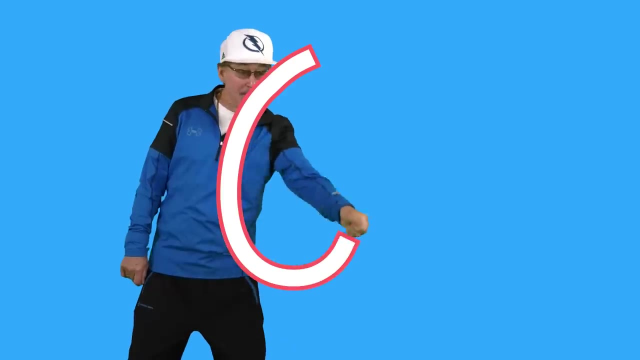 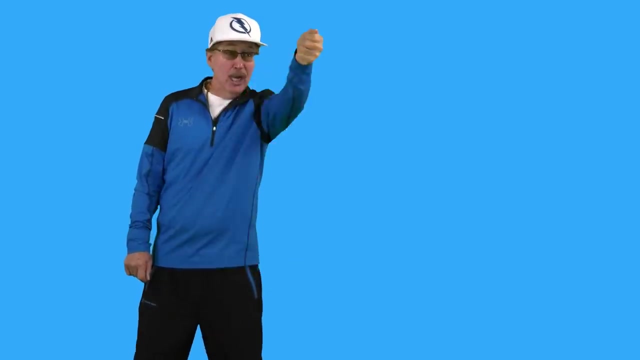 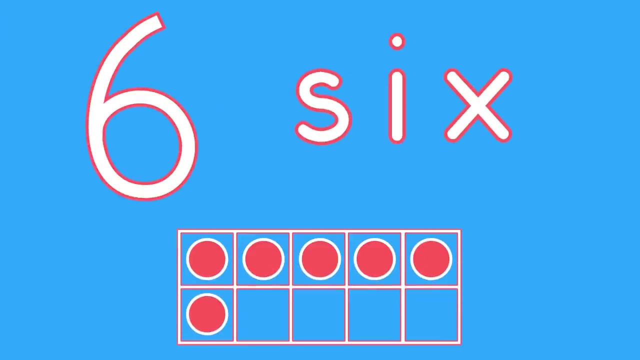 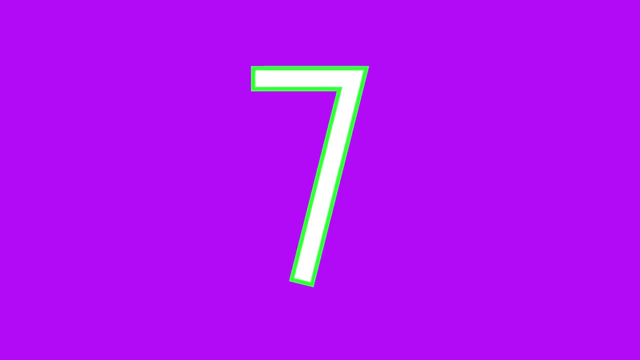 This is number six and you write it like this: Make a curve then loop it quick. Got the scoop. it's number six. Make a curve then loop it quick. Got the scoop. it's number six. S-I-X- number six. S-I-X- number six. This is number seven. this is number seven. 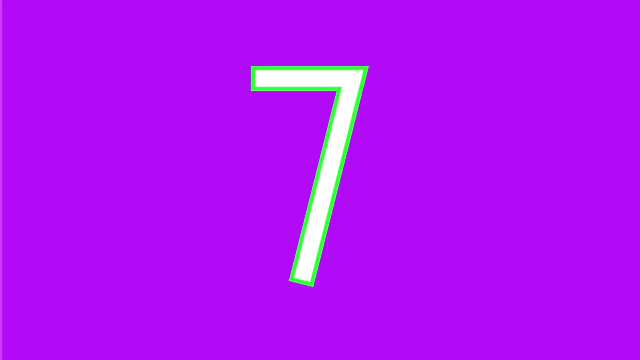 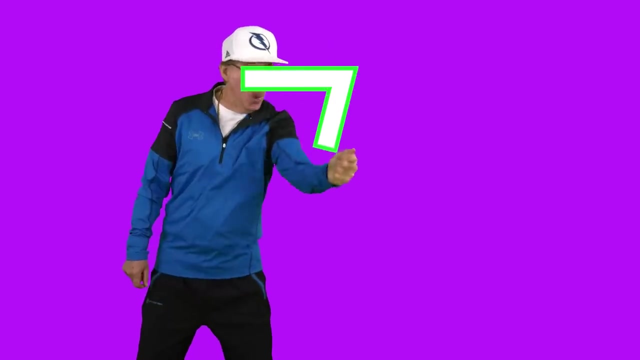 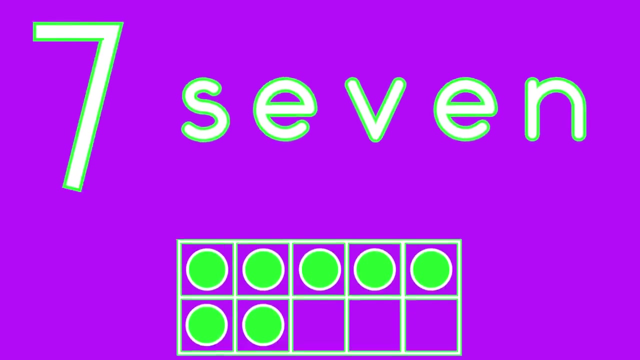 This is number seven and you write it like this: Across the sky, then down from heaven, High to low, it's number seven. Across the sky, then down from heaven, High to low, it's number seven. S-E-V-E-N number seven. S-E-V-E-N number seven. 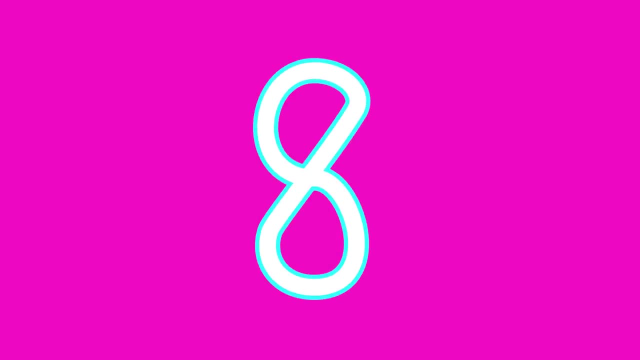 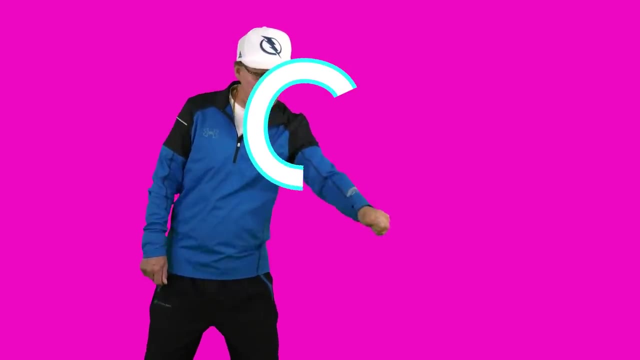 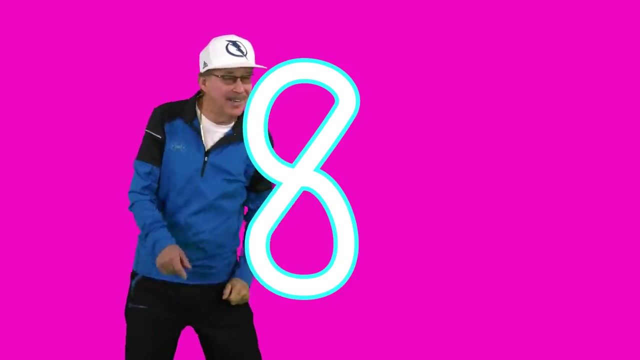 This is number eight. this is number eight. This is number eight and you write it like this: Make an S and do not wait. Curve back up it's number eight. Make an S and do not wait. Curve back up it's number seven. Curve back up it's number eight. 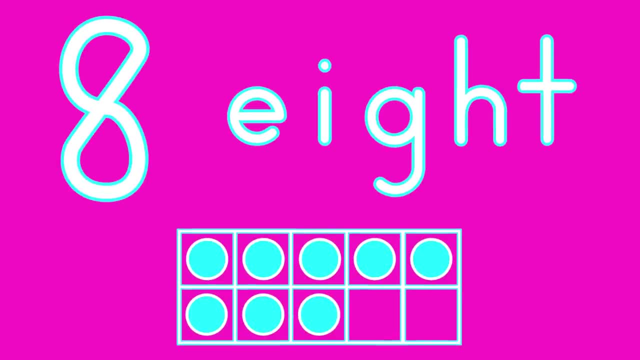 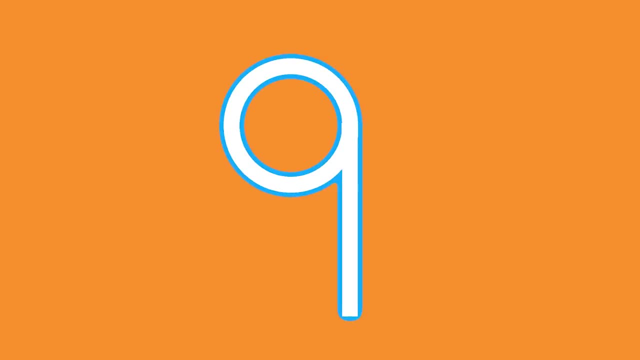 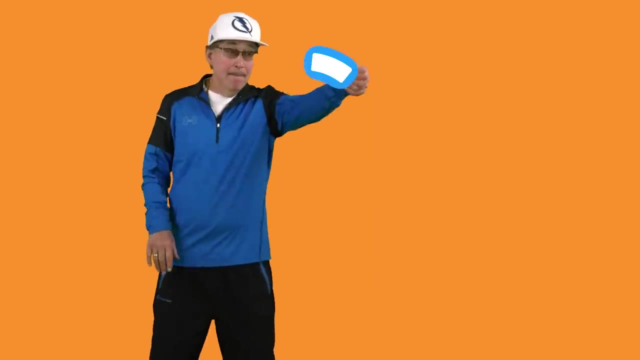 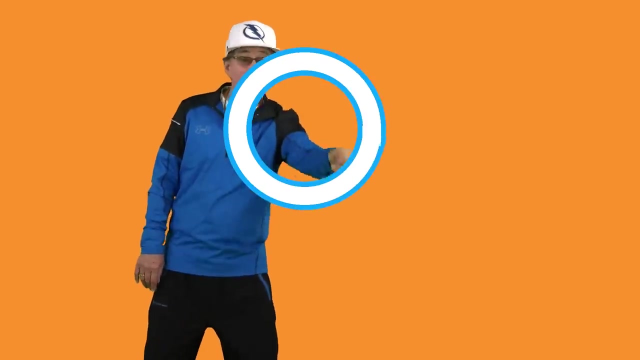 E-I-G-H-T number eight. E-I-G-H-T- number eight. This is number nine. this is number nine. This is number nine. and you write it like this: Make a hoop, then drop a line. After eight, it's number nine. Make a hoop, then drop a line. 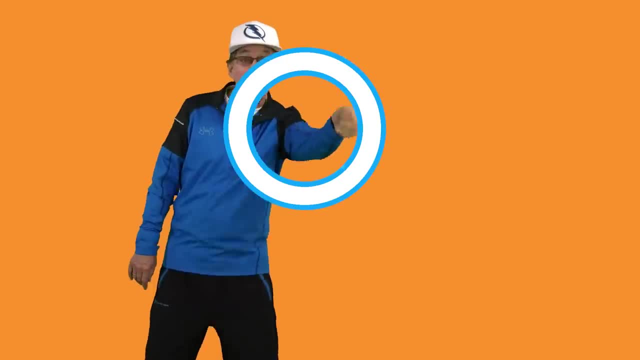 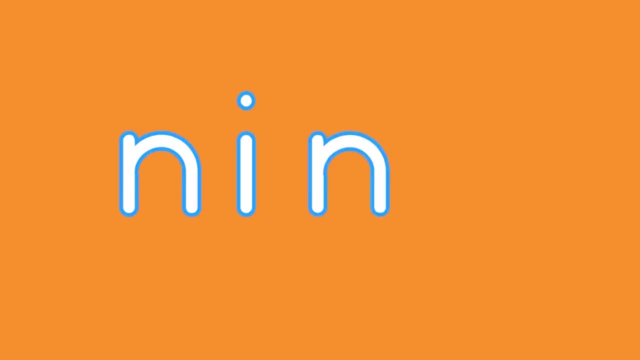 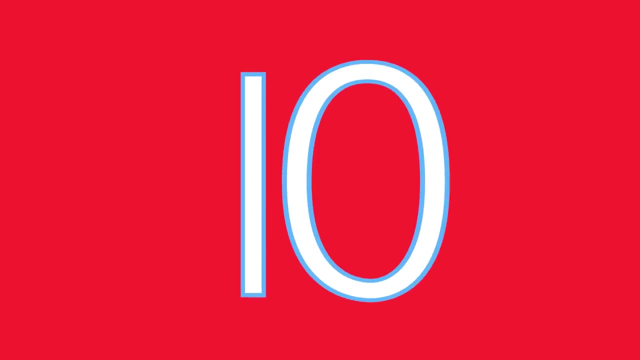 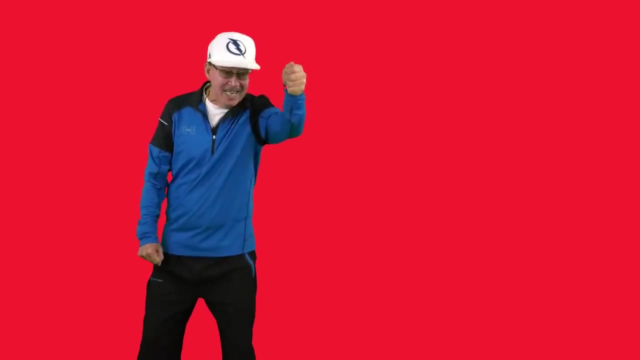 After eight: it's number nine. N-I-N-E number nine. N-I-N-E number nine. This is number ten. this is number ten. This is number ten, and you write it like this: Start at the top and down to the end Circle round left. it's number ten.